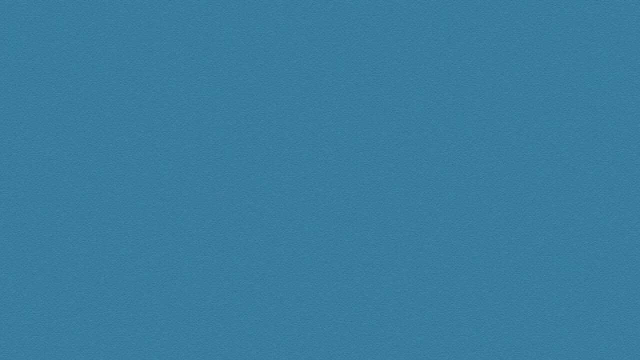 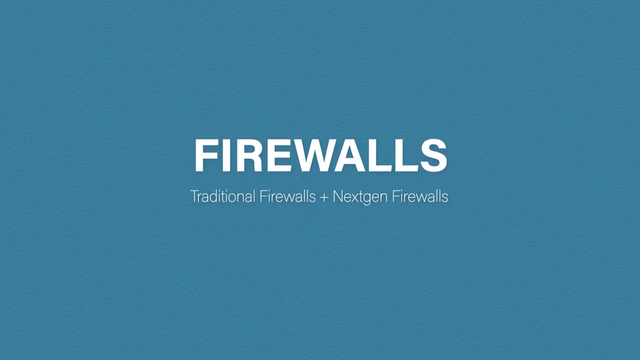 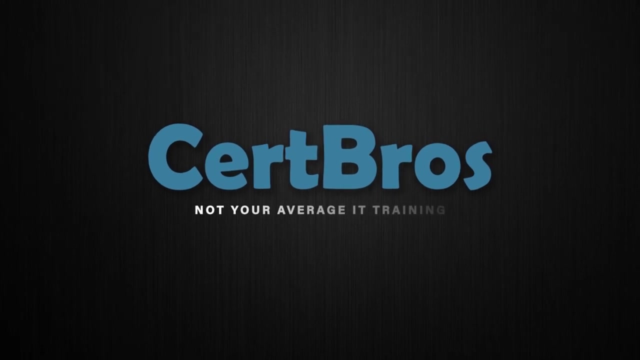 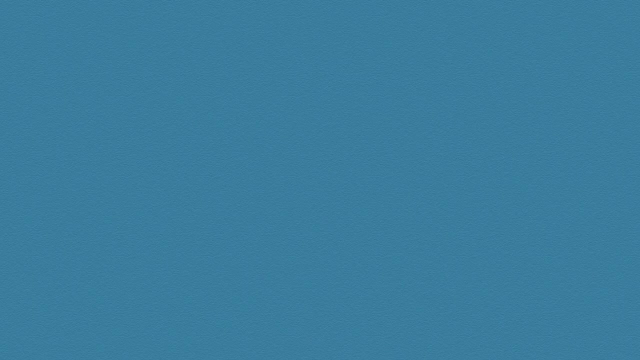 Hey, what's up guys? welcome to Surprose. In this video we're going to be talking about firewalls, What they are, what they do and also the difference between traditional and next-gen firewalls. So first, what is a firewall? If you drive or you're into cars, then you may be familiar with the term. 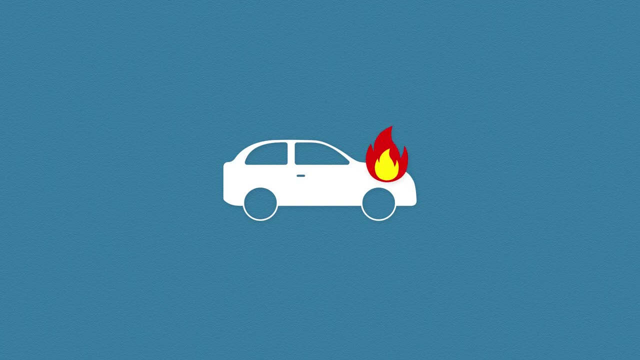 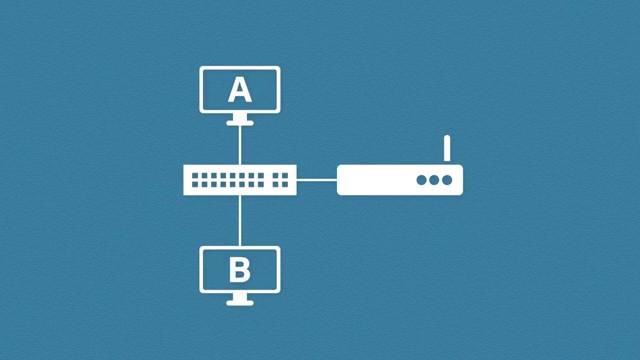 If your engine explodes and catches fire, there is something called a firewall that separates and shields you from the burning hot flames, And network firewalls work in the same way. Let's take this basic network as an example. We have two hosts: a switch and a router. Because you, as a company or as an admin, have control over these devices, policies, antivirus, etc. It's reasonable to consider this as a trusted network, But we have zero control over the devices and networks outside of our own, So it's fair to consider these as 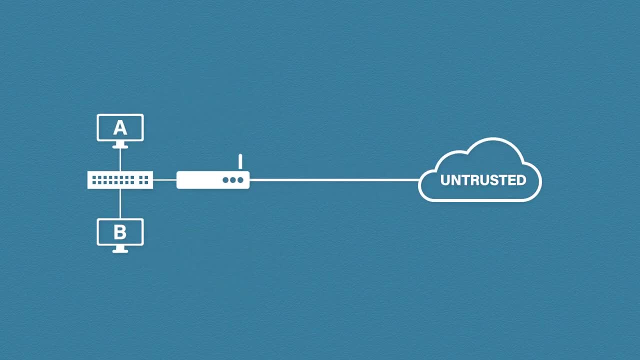 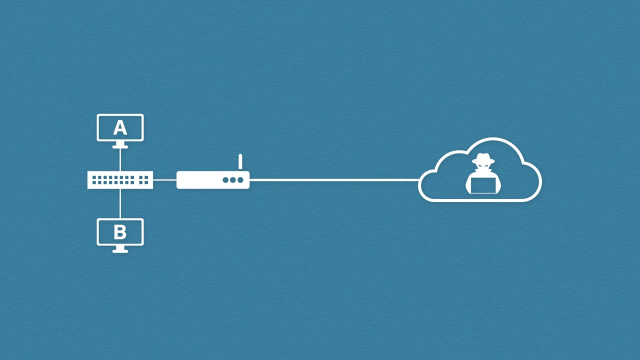 untrusted networks. Now, while most of the world is full of good intentioned, trust worthy people, there are a huge number of bad guys out there looking to take down your systems and get their hands on your hard earned money. With routers generally having minimal security features, 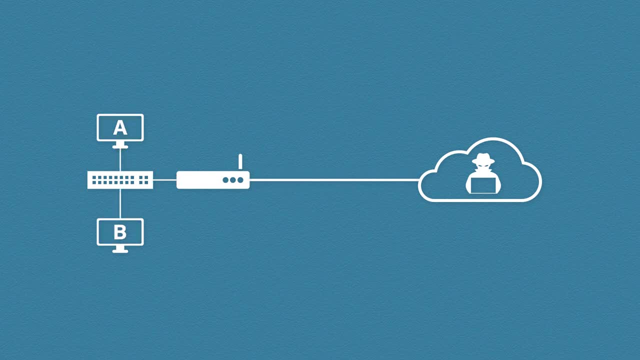 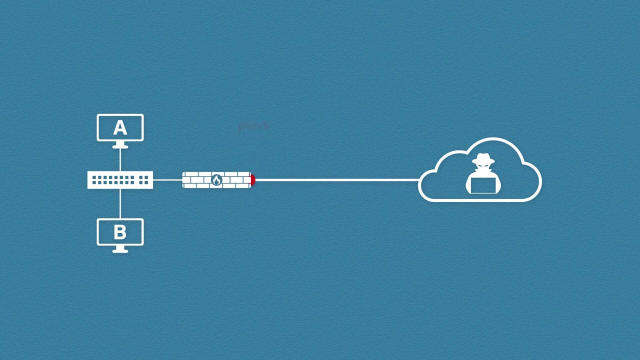 you can quickly be at the mercy of the attackers. This is where firewalls come in. Firewalls are designed to shield and protect your system, our trusted networks, from the untrusted. The idea is that a firewall will block all of the bad traffic from the attackers while at the same time, they'll 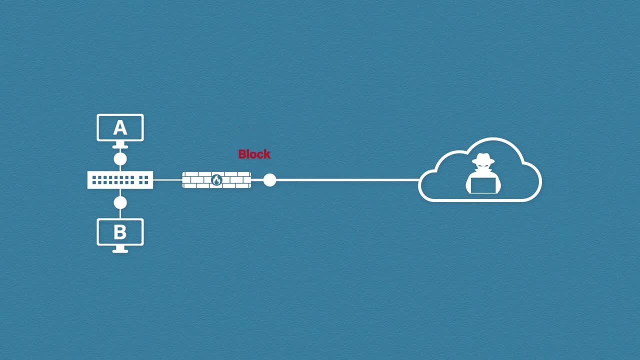 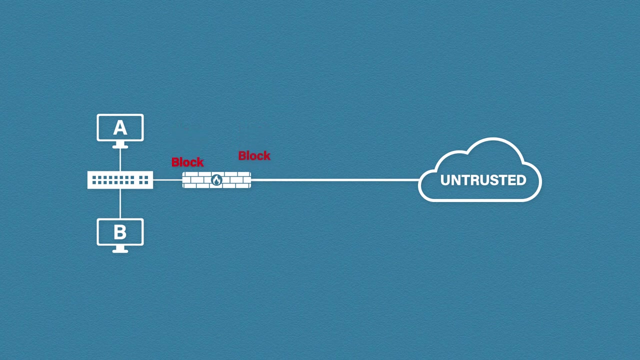 allow normal flow for good traffic. So let's look at how firewalls achieve this. Most firewalls, by default, block everything. It doesn't matter if it's traffic leaving the network or traffic entering the network, Everything is blocked. The way we allow traffic to pass the firewall without being blocked is by 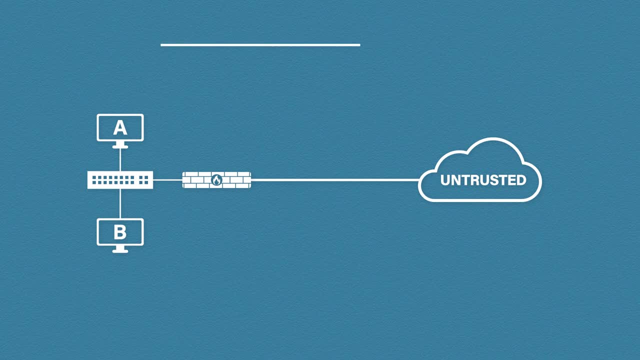 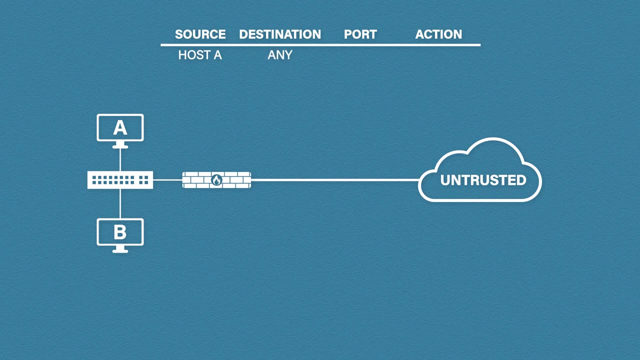 adding something called firewall rules. For example, we may add a rule where the source is host A, the destination is any- because we're not going to add a list of every possible web server- and the port is HTTP or HTTPS, and we'll see how that works. 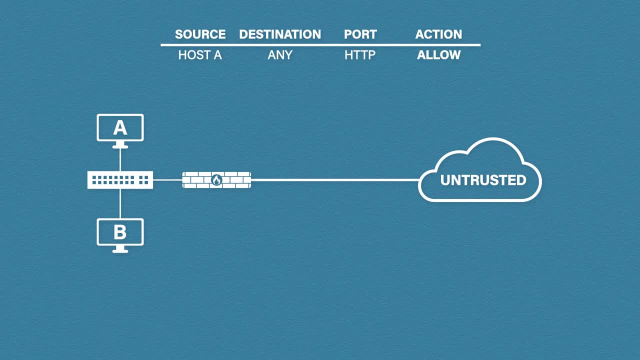 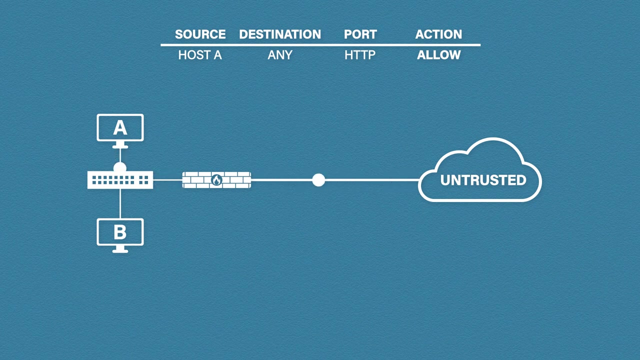 Set the action to allow. The exact firewall rule format will vary from vendor to vendor. Now, when host A sends traffic, the firewall will see this and think: are you from host A? Yes, Are you going to any IP address? Yes, Are you. 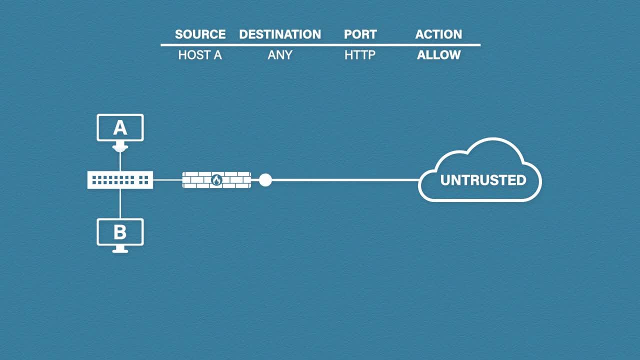 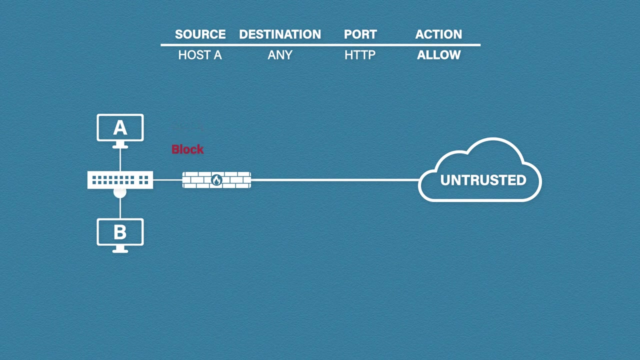 using port HTTP. Yes, Okay, you are allowed, and it lets the traffic through. If host B tries to send traffic, the firewall checks its rules, sees that there are no matching rules and blocks the traffic. So now let's add a rule for host. 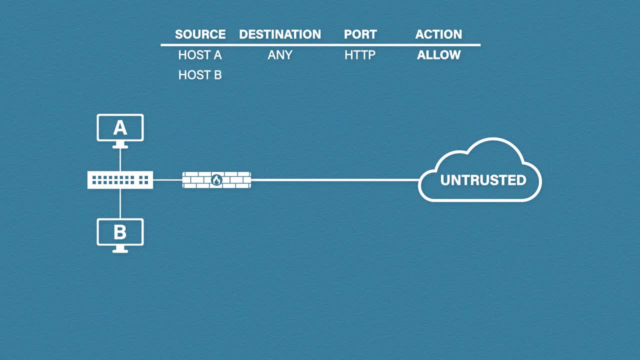 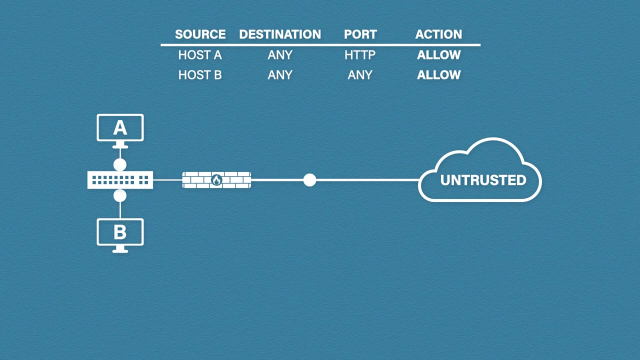 B. Source, host B- Destination: any Port. this time we'll choose any port. Not a recommended rule, but it will do for the sake of the example. Action allow. Now both host A and host B can send traffic through the firewall. So that's traffic leaving the network, but what about traffic entering the? 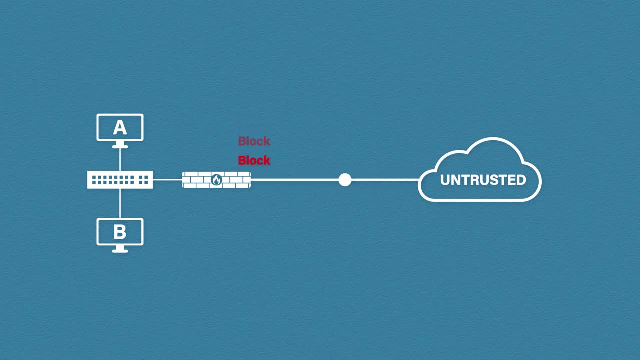 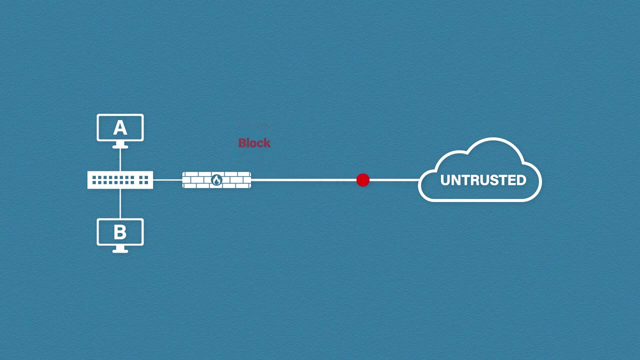 network. Well, it's a good idea to block all traffic from external sources. The only exception is in special cases where you need to open up access for, say, VPN servers, email servers and web servers. But if you do this, they should be tightly controlled by the. 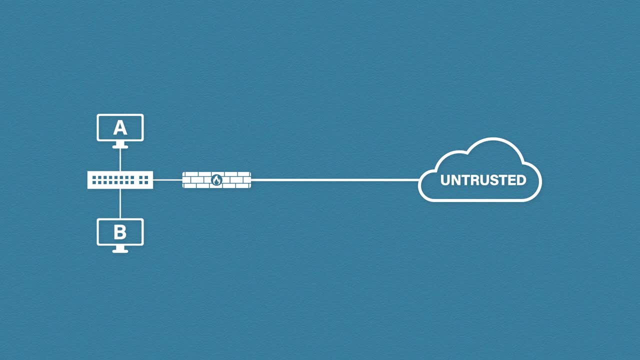 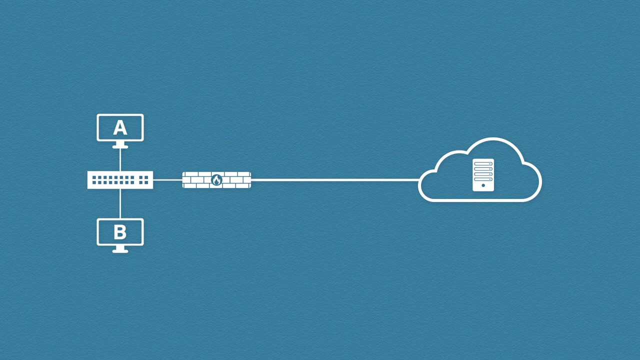 firewall rules. But this poses a bit of an issue for us. Let's say we request a web page, The firewall checks our rules and allows the traffic through. At some point that web server is going to respond right. But if the firewall 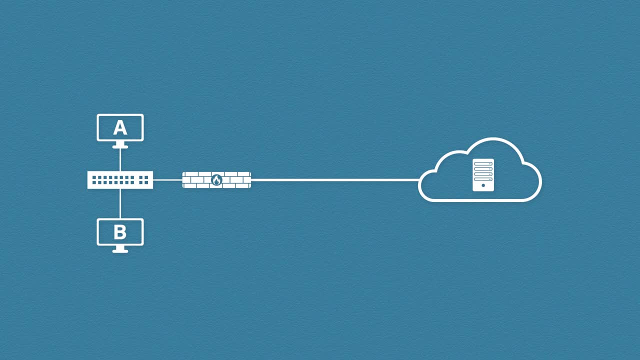 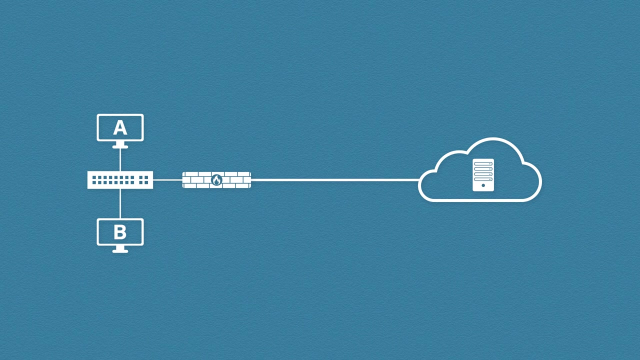 doesn't allow inbound traffic. what does it do? Well, most firewalls are something called stateful firewalls. Stateful firewalls monitor active connections. This means that once outbound traffic has been allowed, the returning traffic is then accepted. This is great, because we don't need to add separate outgoing rules and separate incoming. 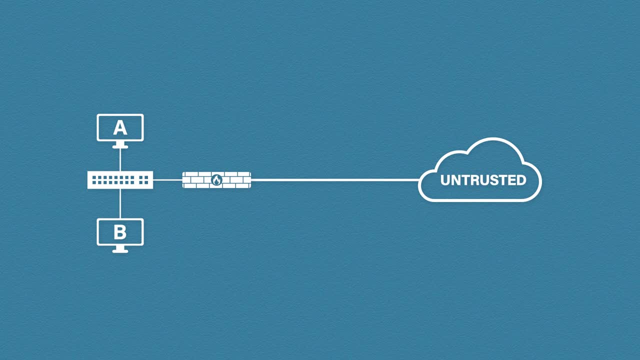 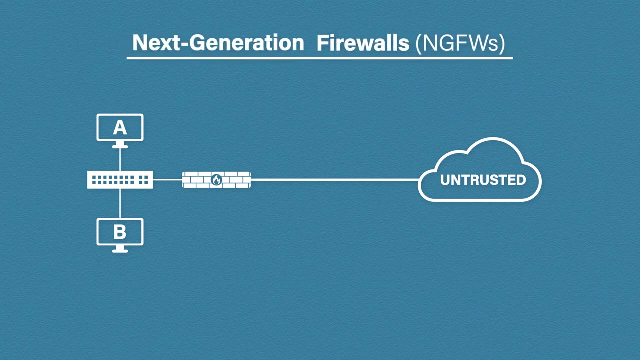 rules. Okay, so everything we've just discussed so far is known as a traditional firewall. It mostly uses firewall rules to block or allow traffic based on a number of things like IP address, port number, etc. Now, next-generation firewalls take the same methods, but then they enhance them. 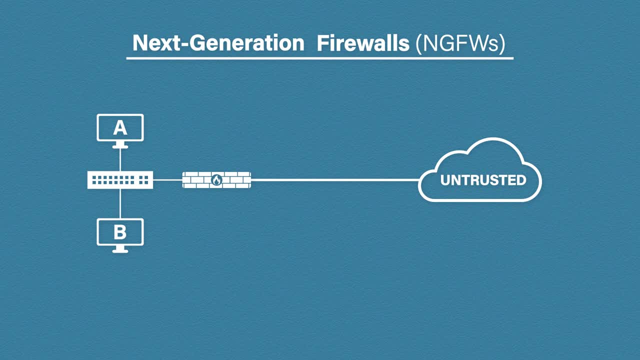 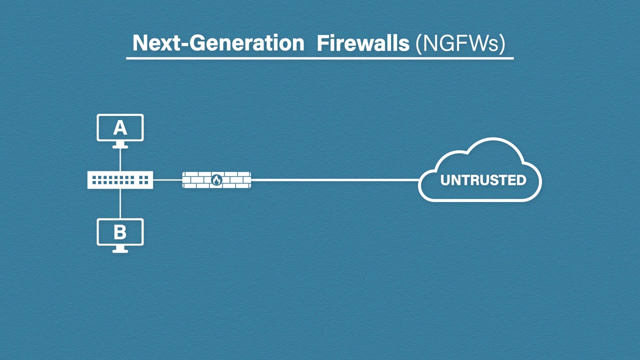 with more in-depth security features. Quick warning: there are a lot of buzz words out there and next-gen firewall is definitely one of them. Different vendors will have slightly different meanings and features to what a next-gen firewall is or what theirs does, But generally speaking, this is what a 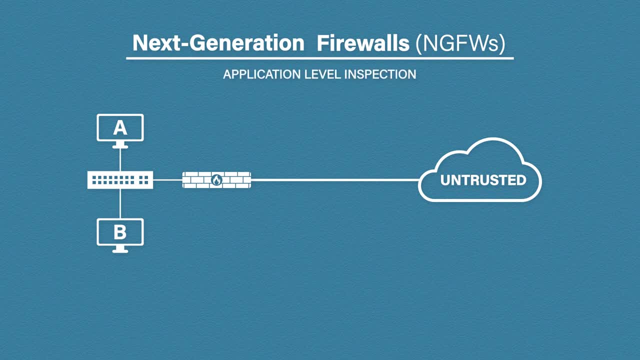 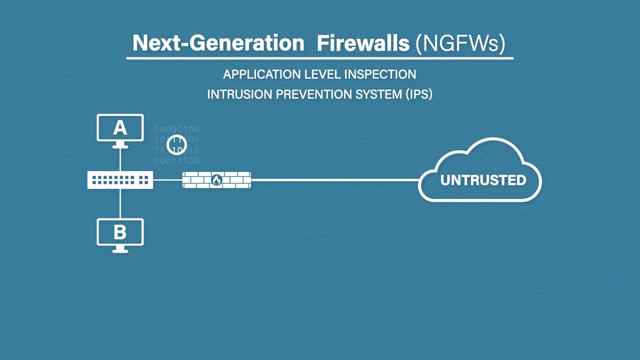 next-generation firewall should include Application level inspection So the firewall can identify and block risky application traffic Intrusion prevention systems, or IPS. IPS will inspect the contents of the traffic and look for patterns or signatures. It's looking for malicious or malware related. 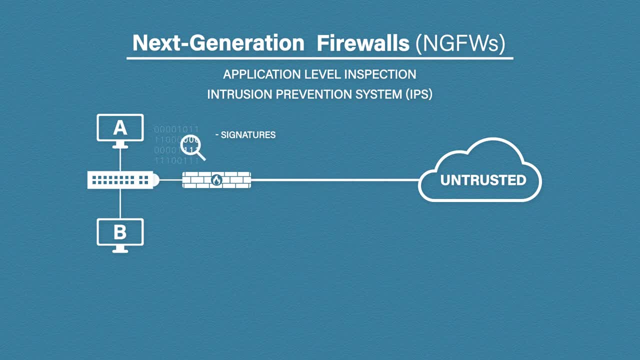 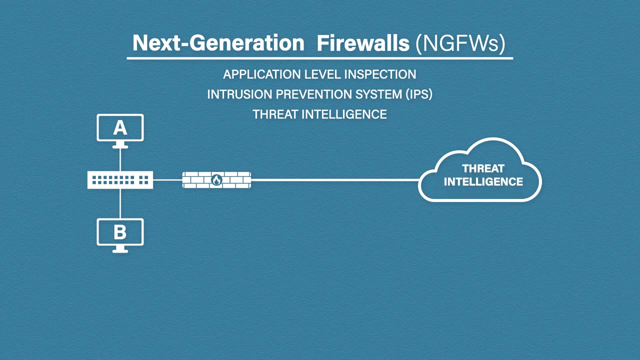 traffic. IPS can also detect anomalies and unusual traffic. External threat intelligence: Next-generation firewalls can update themselves from external threat intelligence sources, So if a brand-new attack has been identified, the vendor can update the firewalls threat intelligence to be able to identify this new emerging threat. 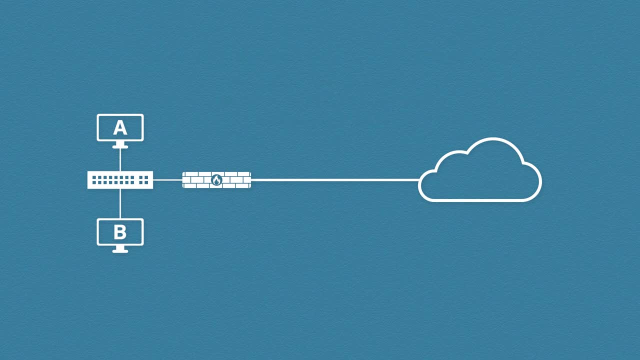 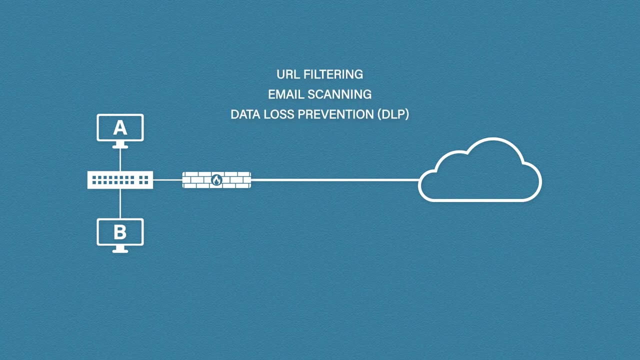 There are a huge number of features that firewalls can offer, Things like URL filtering, email search and email access. There are a huge number of features that firewalls can offer, Things like URL filtering, email scanning, data loss prevention or DLP, and the list goes on and on Firewalls that. 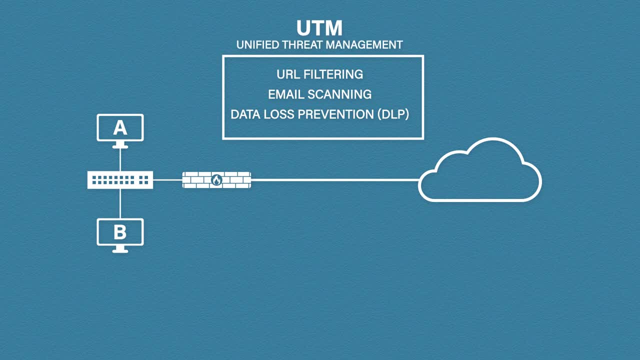 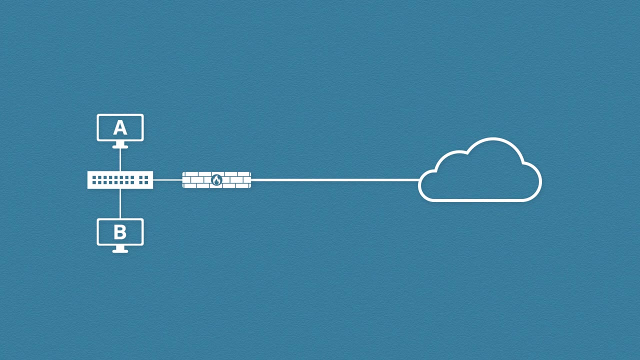 have. features like these are often known as UTMs or unified threat management. The idea is you have a single appliance that unifies all of these security features. So that is how a network firewall works, But you may have seen another type. Computers can also have software-based firewalls.